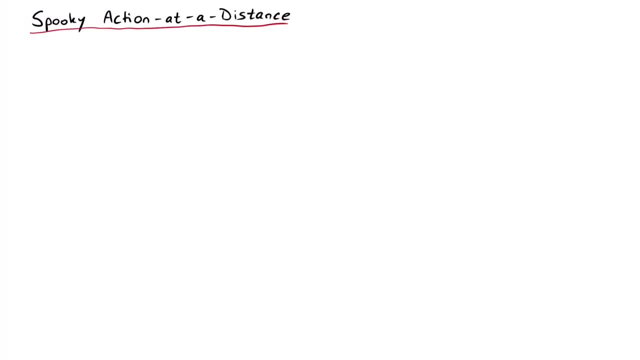 Spooky action at a distance. Albert Einstein used these words to express his disbelief about a certain interpretation of quantum mechanics. In this video, we will take a look at entanglement and the Einstein-Podolsky-Rosen paradox and see whether physics is really spooky or not. 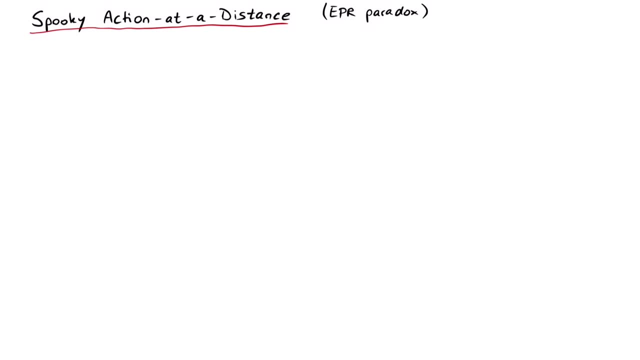 The fascinating, although confusing, thing about quantum mechanics is that the wavefunction psi does not uniquely determine the outcome of an experiment. It only provides us with probabilities of the different outcomes. So how does it happen that one particular outcome is a result when we perform a measurement? One possible way to answer this would be that the wavefunction already knew. 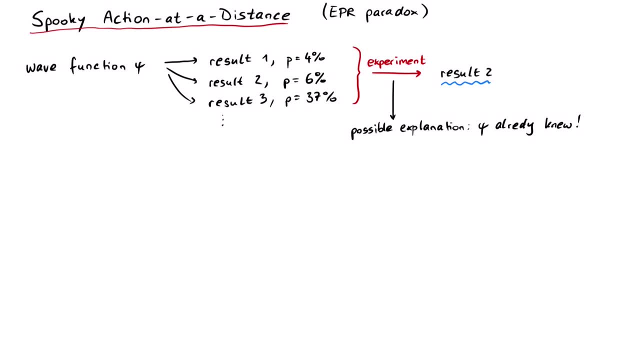 which outcome would be the result before we even measured it. If this were correct, then the quantum mechanics as we have it today would be an incomplete theory. If the wavefunction really knows the result before the measurement, why is this not accounted for in the theory? Maybe we should introduce an additional parameter. 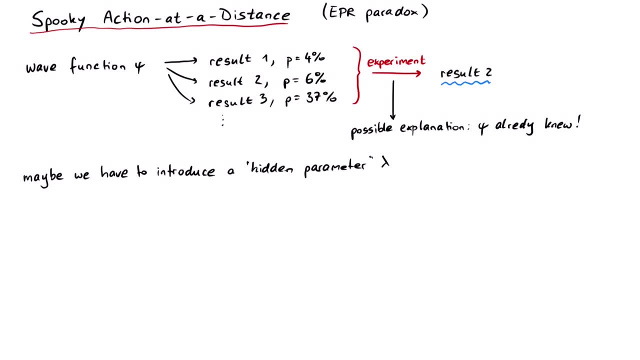 Call it lambda, which contains the necessary information that determines the outcome. So two wavefunctions that might look the same now could really be distinguished by their hidden parameter, lambda. And by using lambda in our calculations we should be able to precisely predict the outcome of a quantum mechanical measurement. No more probabilities. 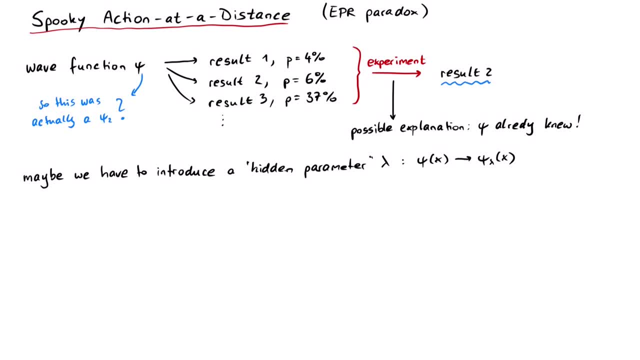 Including this hidden parameter, lambda, apparently solves our question. Therefore, not accounting for lambda makes our current theory of quantum mechanics incomplete. In 1935, Einstein, Podolsky and Rosen designed a thought experiment in order to prove that quantum mechanics is indeed incomplete and that we need to refine it somehow. 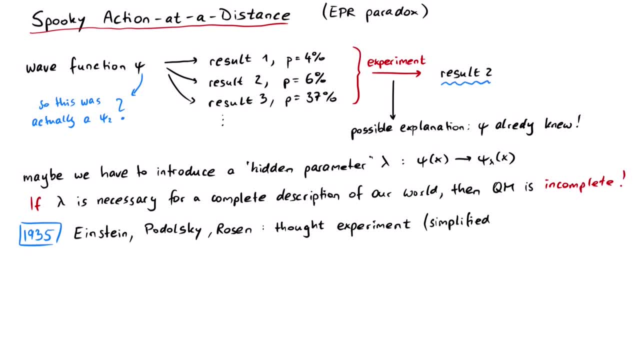 For this video. we will consider a simplified version of their thought experiment, introduced by David Bohm. We consider the decay of a neutral pion into an electron and a positron. In the rest frame of the pion, the electron and positron move apart in exact opposite. 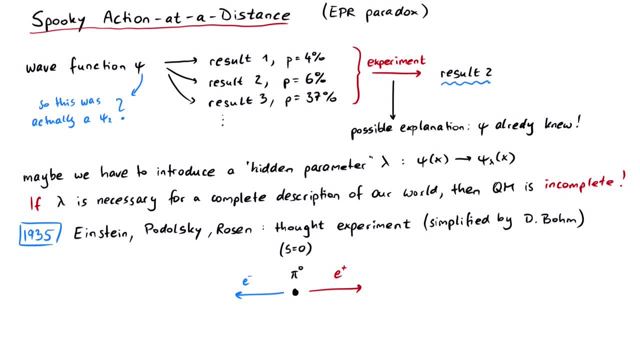 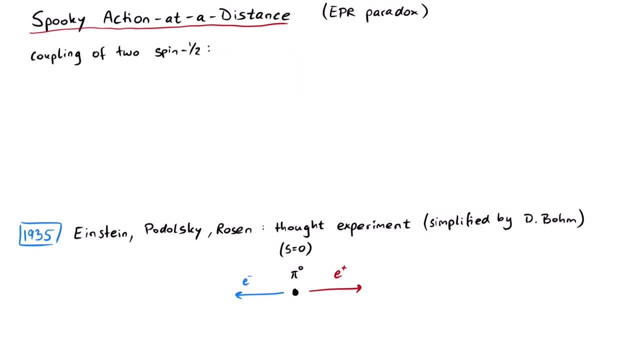 directions. Since the pion has spin zero, the spins of the electron and the positron must point in opposite directions. Mathematically we can express the composite system of two spins like this: These three expressions correspond to the total spin. one case and this one corresponds. 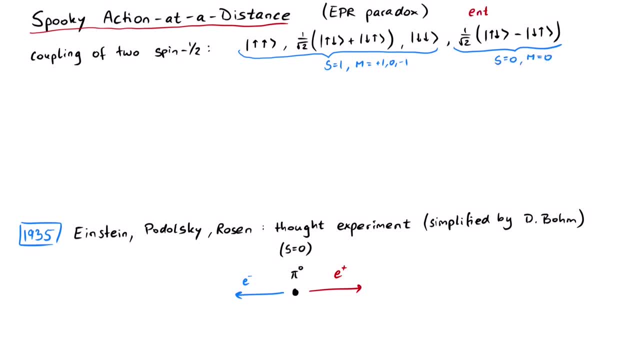 to the total spin zero case. This is a so-called entangled state. The definition of an entangled state is that it cannot be written as the product of two states And if we measure the first spin, let's say that's the spin of the electron as up. 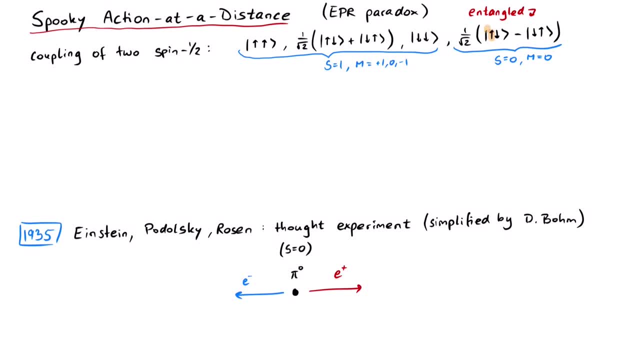 then there is no other possibility than that the spin of the positron must be down. Here comes the tricky part. Let's assume that after the pion decays, we let the electron and the positron fly far away, really far, 10 meters, 10 kilometers, 10 light. 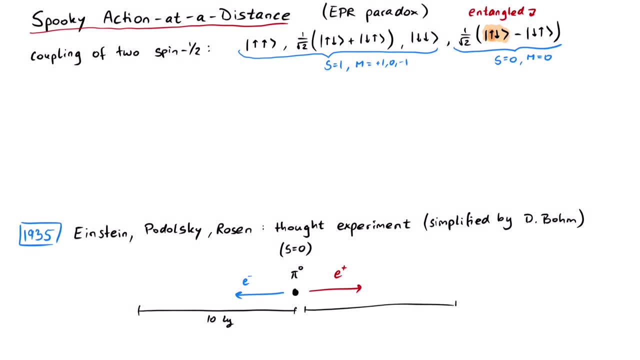 years. If we measure one spin, then we know that someone 20 light years away will 100% measure the current distance. If we measure one second behind, then we know that the second spin is going to limit the speed of light. With this we can himself call all the three of 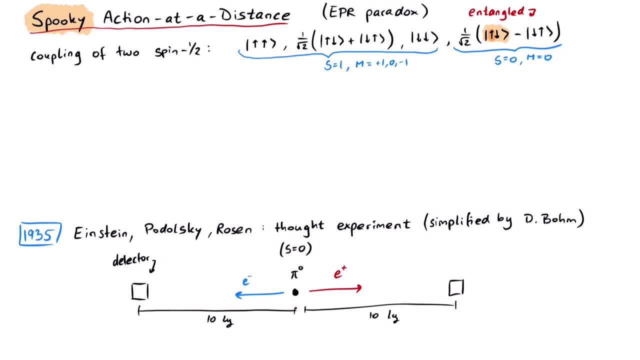 these information possibilities and we can draw the whole equation out here. So we can assume that the first spin is the product of a speed of light, the second is the product of a speed of light, And that's the idea of the spin of a particle. Then we can also: 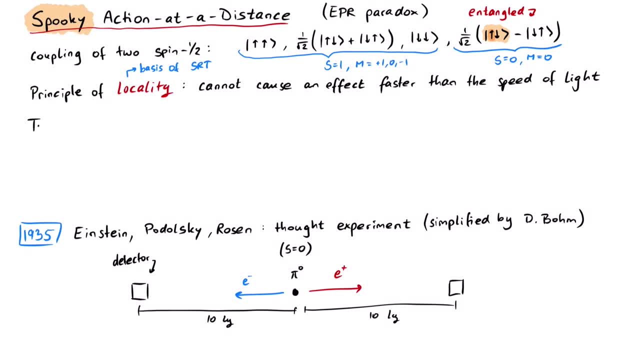 has a way to communicate faster than light. So at this point we basically have two options. One, that there are indeed hidden variables that already decide the spin the moment the pion decays. This way no information is ever transmitted. both particles already knew in. 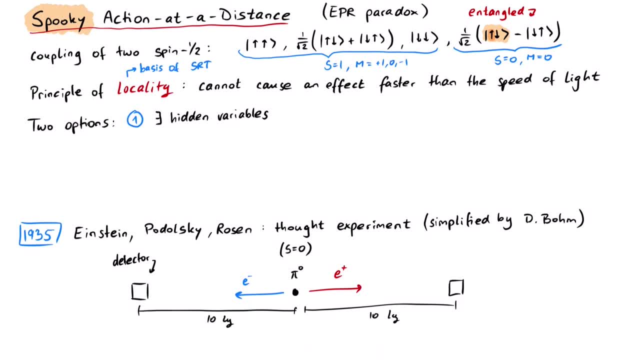 which direction their spins would point during the experiment Or two, that nature is simply non-local and that there is stuff that happens faster than the speed of light. The answer came almost 30 years later, delivered by John Stuart Bell and his famous inequalities. 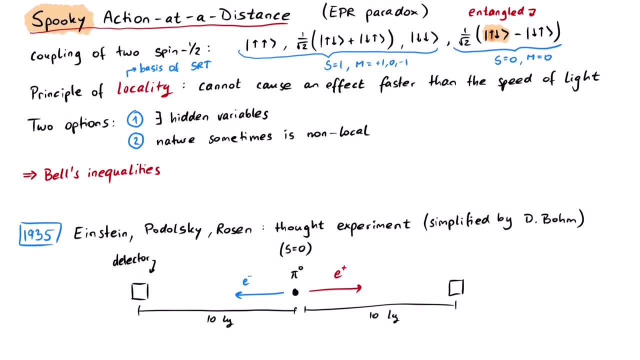 They absolutely deserve a video on their own. so to keep things short, the argument goes like this: If Bell's inequalities hold true, then we cannot have any hidden parameters and nature really behaves non-locally. If Bell's inequalities fail, then we have to modify our theory of quantum mechanics and introduce lambda somewhere. 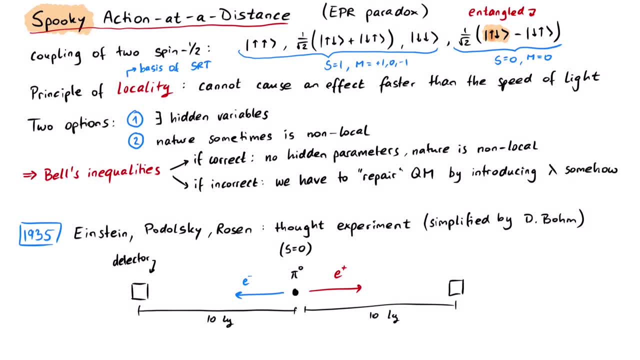 There are a few ways to do this. The first way to do this is to use the theory of quantum mechanics. There are a few ways to do this. The first way to do this is to use the theory of quantum mechanics. There have been many, many experiments to verify Bell's inequalities and so far,